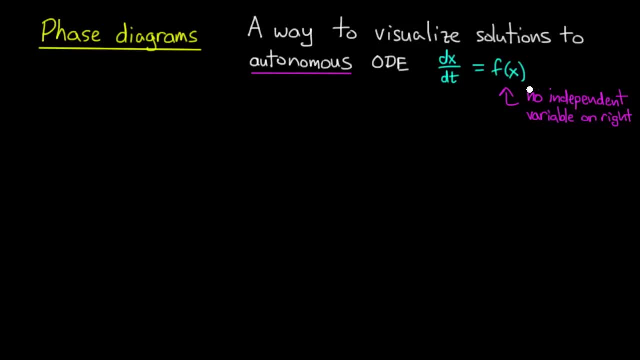 not include the independent variable. So the independent variable is not used in the definition of the differential equation. I'll show you how to construct phase diagrams through an example. So let's consider the differential equation: dx. dt equals x times 1 minus x. This 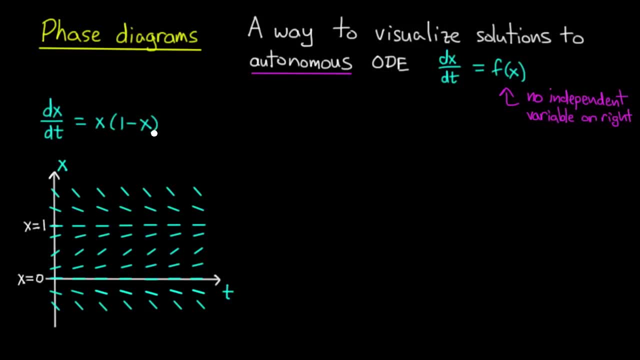 is autonomous because the independent variable t does not appear on the right hand side. Now, phase diagrams are kind of related to slope fields, so I'll start by drawing the slope field for this differential equation, as I've done here. I'll remind you how. 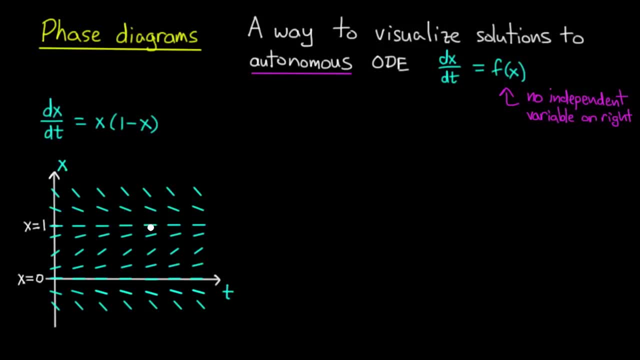 to draw this slope field. You pick a point t x in the t x plane and you imagine that you have a slope field x and a minus x and you draw a slope field. Here's the solution. passing through that point, The tangent line to that solution, will have slope dx, dt. 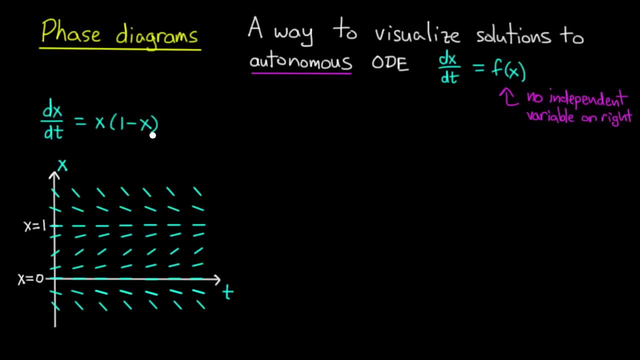 but the equation says that dx dt is the same as x times 1 minus x. So if you go to that point and you draw on a little line which has slope x times 1 minus x, then that will be a tangent line to the 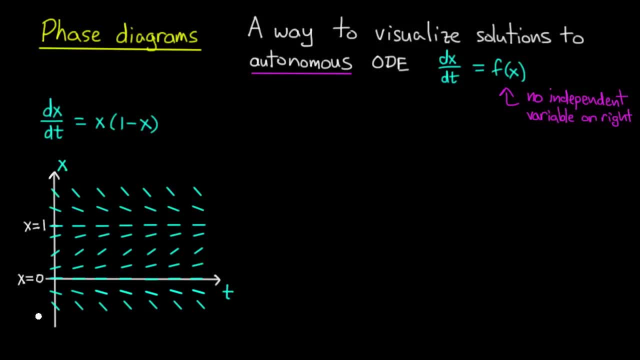 solution. I do that for a bunch of points in this plane, and I begin to get a picture of how the solutions will flow. Now notice a special property of this slope field. Because the equation is autonomous, the right hand side does not depend on t, and so the slope field will not change as 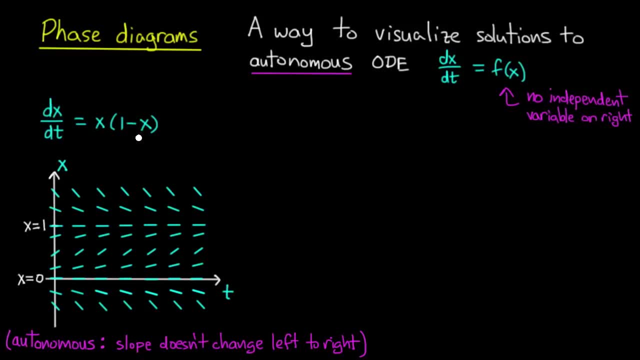 I move from left to right. If I choose a particular x value and I evaluate the slope by evaluating x times 1 minus x, then I can move from left to right. In other words, I can change the value of t and I still have the same slope. Phase diagrams take special advantage of this: left to right. 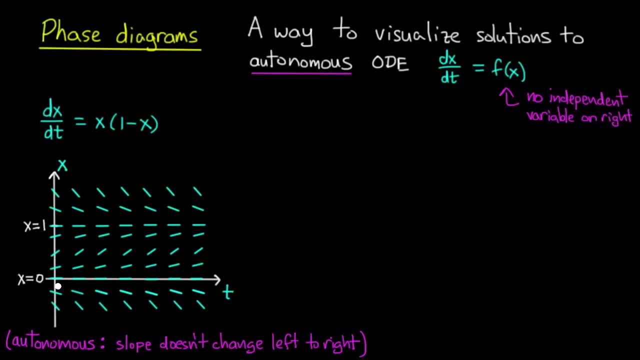 symmetry in the slope in order to collapse this two-dimensional picture down into a single line. So here's our phase diagram, At least the beginning of it, And since it's a line, we'll call it a phase line. Now, before we draw any more of this phase line, let's sketch in a few solutions to this differential. 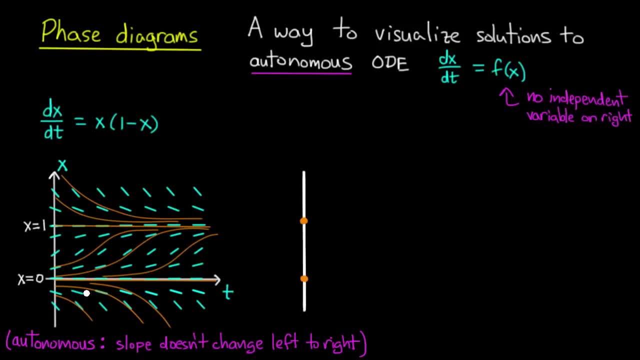 equation. So I go with the flow of the slope field and sketch in some solutions. in orange Now notice we have two particular solutions which are special And those are the solutions x of t equals 1 and x of t equals 0. Constant solutions: Those correspond to the points where dx, dt is 0,. 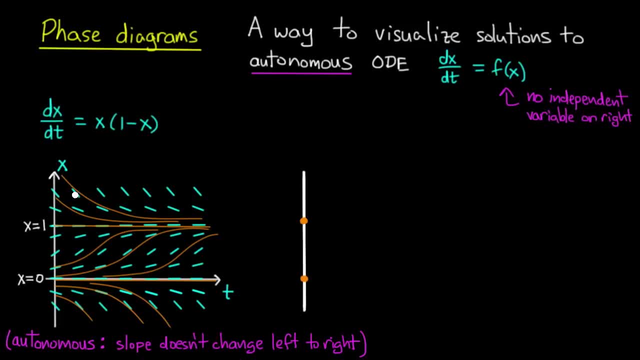 and the solution is not constant. So we have x of t equals 1 and x of t equals 0. Constant solutions: Those correspond to the points where dx, dt is 0, and the solution is not changing. For all of the other solutions it will change with time, And so I mark those guys in here by filling in just an. 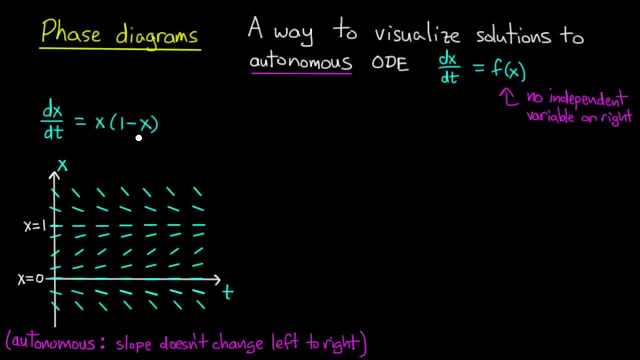 move from left to right. If I choose a particular x value and I evaluate the slope by evaluating x times 1 minus x, then I can move from left to right. in other words, I can change the value of t and I still have the same slope. Phase diagrams take special advantage of this: left to right. 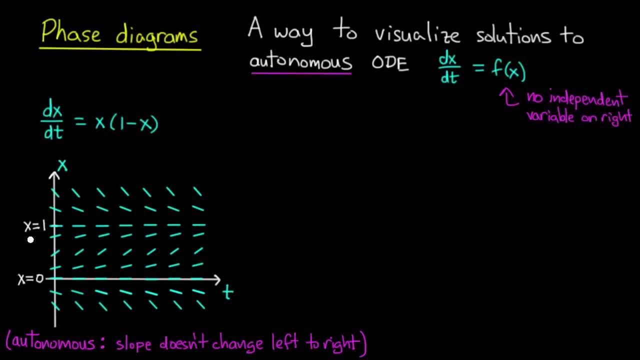 symmetry in the slope in order to collapse this two-dimensional picture down into a single line. So here's our phase diagram, at least the beginning of it, and since it's a line, we'll call it a phase line. Now, before we draw any more of this phase line, let's sketch in a few solutions to this differential. 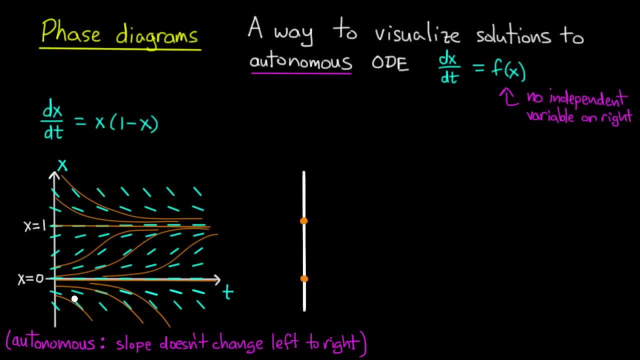 equation. So I go with the flow of the slope field and sketch in some solutions. in orange Now notice we have two particular solutions which are special and those are the solutions x of t equals 1 and x of t equals 0,. constant solutions: Those correspond to the points where dx, dt is 0,. 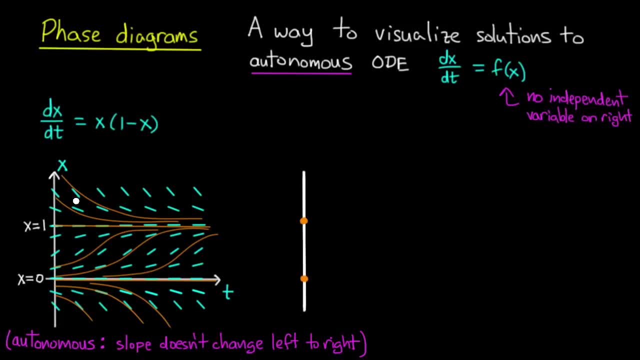 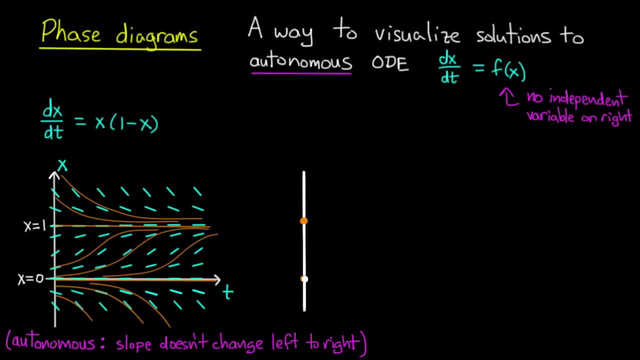 not changing much. For all of the other solutions, it will change with time, and so I mark those guys in here by filling in just an orange circle corresponding to the points x equals 0 and x equals 1.. These are the guys where dx dt is is 0. The solutions are not changing. 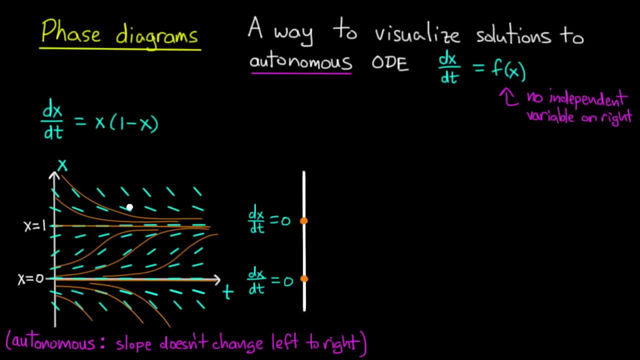 What about elsewhere on this phase line? Well, if I start out above x equals 1,, then my solution will decrease. If I start out between x equals 0 and x equals 1,, then my solution decreases and there will just be characters inside thegendext equations. 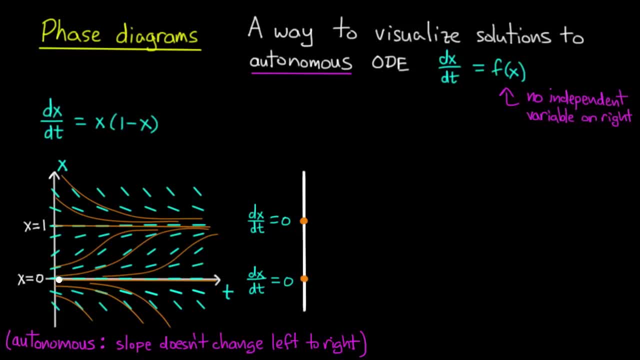 x equals 1,, my solution will increase. If I start out below x equals 0,, then my solution will decrease. So that corresponds to different signs for the derivative. Above x equals 1, dx dt by this formula is negative. Between x equals 0 and x equals 1,, again by this formula. 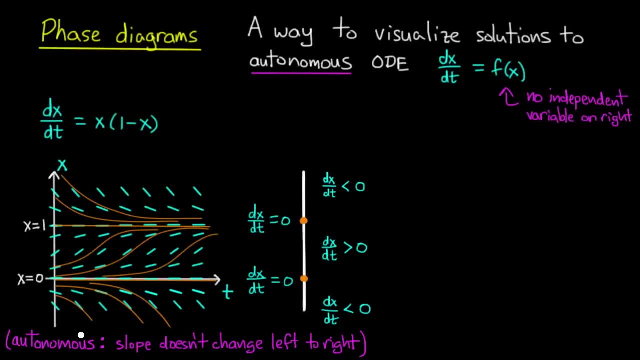 dx dt is positive And below x equals 0, dx dt is negative. So as a shorthand we can mark in those signs on our phase line by drawing little arrows At these orange points. the solution will stand still. so I just draw a little circle Now in between the orange. 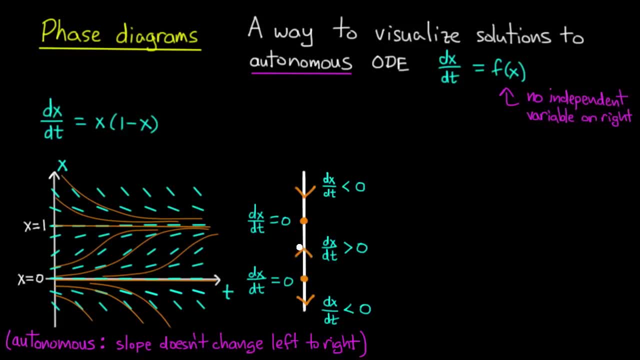 points say: right here, the solution will increase. so I draw a little arrow going up Above the top orange point at x equals 1, the solution will decrease. so I draw an arrow going down Now. likewise for below, x equals 0, I draw an arrow going down And that's. 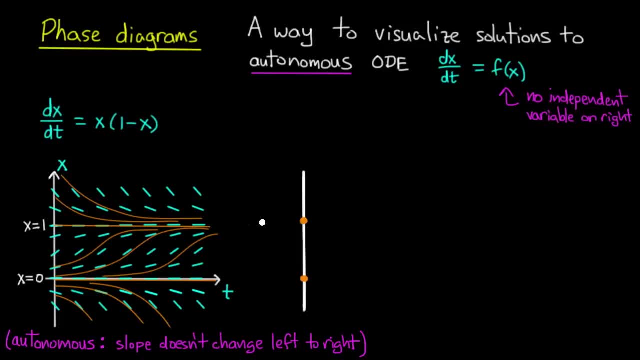 orange circle corresponding to the points x equals 0 and x equals 1.. So these are the guys where dx dt is 0. The solutions are not changing. What about elsewhere on this phase line? Well, if I start out above x equals 1, then my solution will decrease. If I start out between x equals 0 and x, 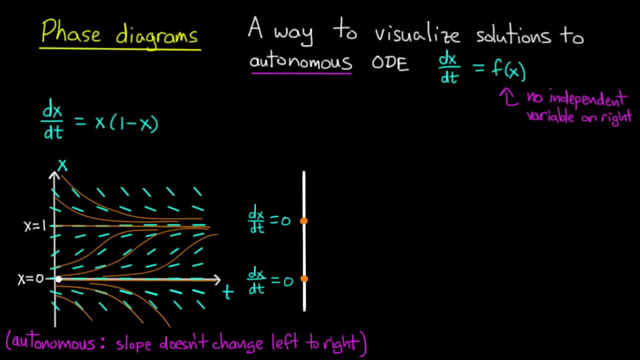 x equals 1,, my solution will increase. If I start out below x equals 0,, then my solution will decrease. So that corresponds to different signs for the derivative. Above x equals 1, dx dt by this formula is negative. Between x equals 0 and x equals 1,, again by this formula. 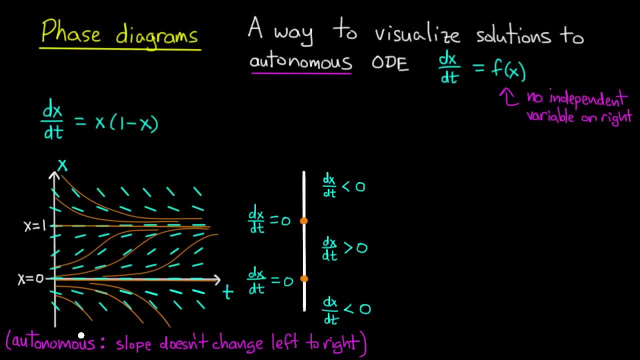 dx dt is positive And below x equals 0, dx dt is negative. So as a shorthand we can mark in those signs on our phase line by drawing little arrows At these orange points. the solution will stand still. so I just draw a little circle Now in between the orange. 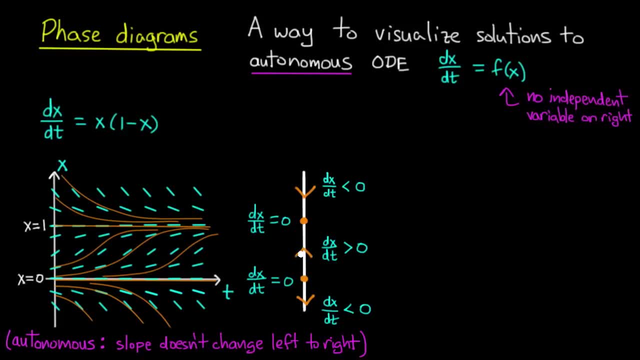 points say: right here, the solution will increase. so I draw a little arrow going up Above the top orange point at x equals 1, the solution will decrease. so I draw an arrow going down Now. likewise for below, x equals 0, I draw an arrow going down And that's. 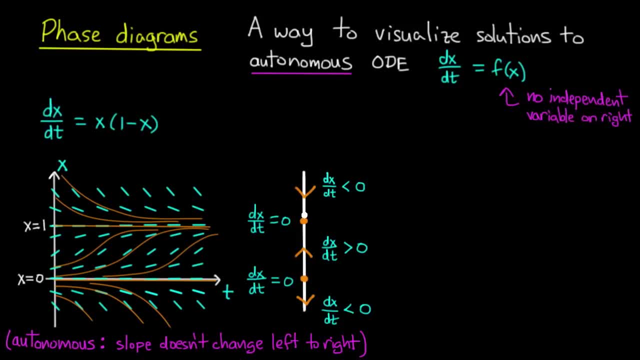 it. That's our phase line. So we have a line with dots to indicate where the solution is standing still and arrows to indicate where it's moving and in which direction it's moving. So let me give you a little vocabulary that will help you talk about the phase line. 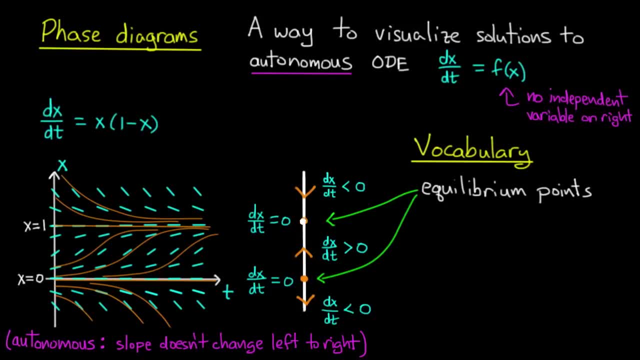 And the first thing is that these points where the solution is standing still, these are called equilibrium points. In our case, it's x equals 1 and x equals 0. Equilibrium meaning that the solution is not changing. Now these equilibrium points have different properties. 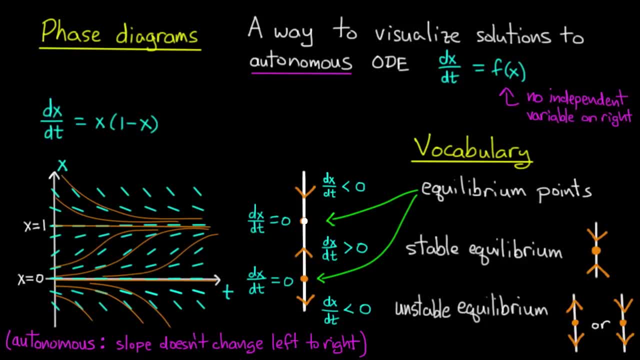 And this equilibrium point at x equals 1 and x equals 0 is the point where the solution is not changing. It's a stable equilibrium point, And we call it stable because both of the arrows are pointing in. So you imagine that if you were to start off close to x equals, 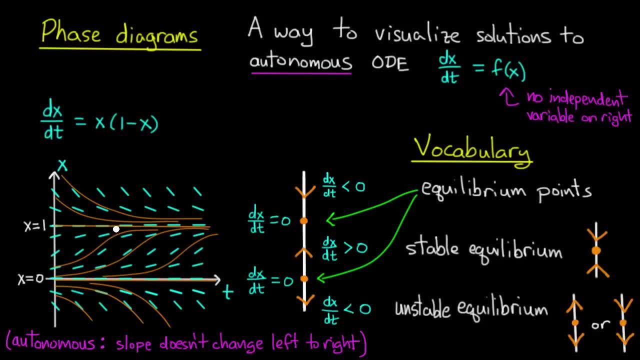 1, either above it or below it. you would tend toward x equals 1.. And that's what makes it stable. It's like the bottom of a valley And the other point. the arrows are pointing away from that equilibrium, And so it's called an unstable equilibrium. You imagine it like. 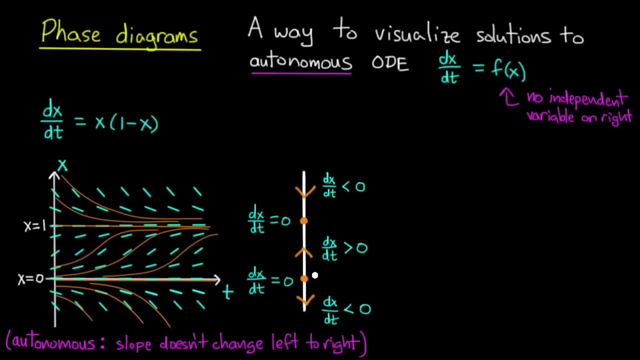 it. That's our phase line. So we have a line with dots to indicate where the solution is standing still and arrows to indicate where it's moving and in which direction it's moving. So let me give you a little vocabulary that will help. 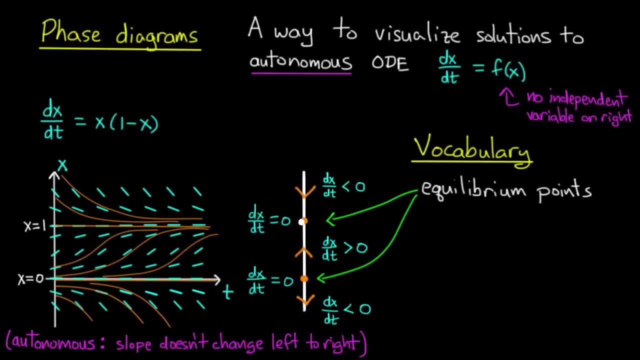 you talk about the phase line And the first thing is that these points where the solution is standing still, these are called equilibrium points. In our case, it's x equals 1 and x equals 0.. Equilibrium meaning in that the solution is not changing. Now, these equilibrium, 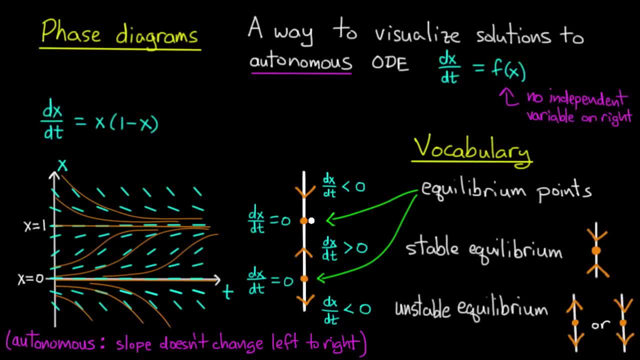 points have different properties, and this equilibrium point is x equals 1, whatever one we call a stable equilibrium, and we call it stable because both of the arrows are pointing in. so you imagine that if you were to start off close to x equals one, either above it or below. 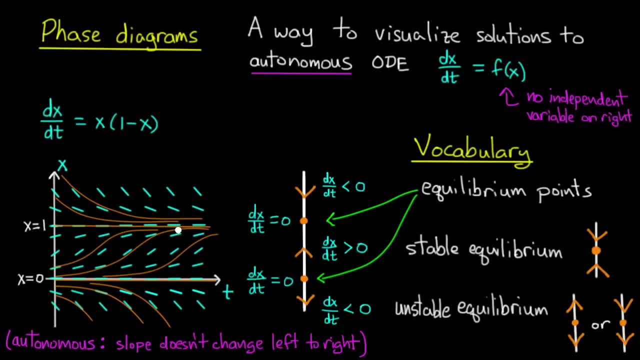 it you would tend toward: x equals one, and that's what makes it stable. it's like the bottom of a valley and the other point, the arrows are pointing away from that equilibrium, and so it's called an unstable equilibrium, you imagine, like the top of a mountain. so if i start out, anywhere near, x equals. 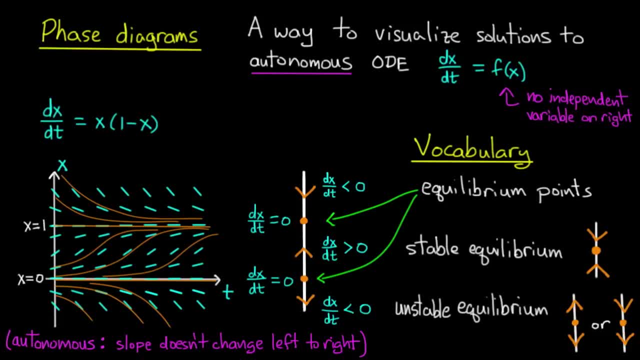 0, then i will move away from x equals 0.. similarly, if i were to concoct a differential equation which had this as part of its phase diagram, where an arrow was pointing in and an arrow was pointing out, i would also call that unstable, because it is not stable. now i have a task for you. 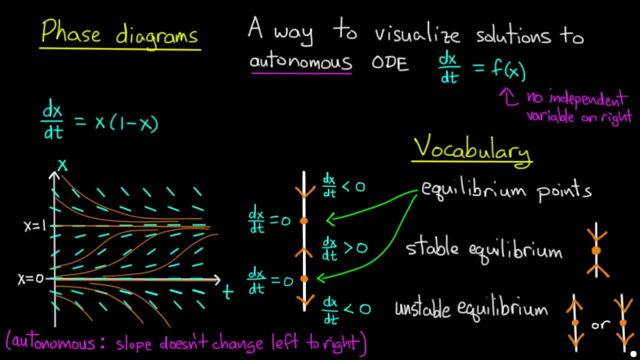 since this type of unstable equilibrium did not appear in our example, come up with an example of an equation that exhibits this type of unstable equilibrium, and that is one arrow going into the equilibrium and one arrow going out. Now, after you figure out how to do that, I have 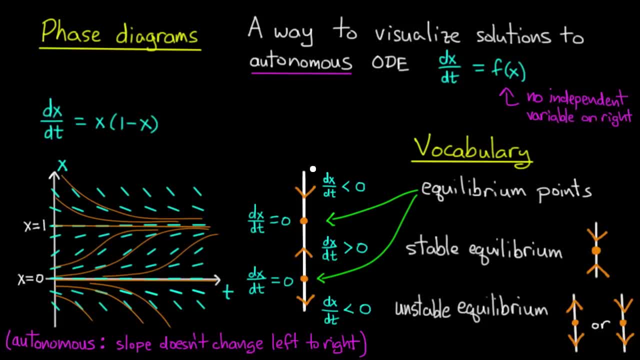 a question: Is there any phase line, any configuration of stable and unstable equilibria which could not occur as the phase line for a differential equation? In other words, can I glue together a whole bunch of these guys in some line which could not possibly be the phase line for a 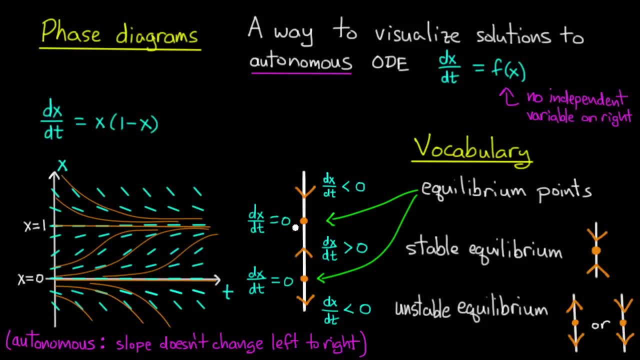 differential equation, Or is it true that any picture I draw, I can come up with an example of a differential equation which has that picture as its phase line?